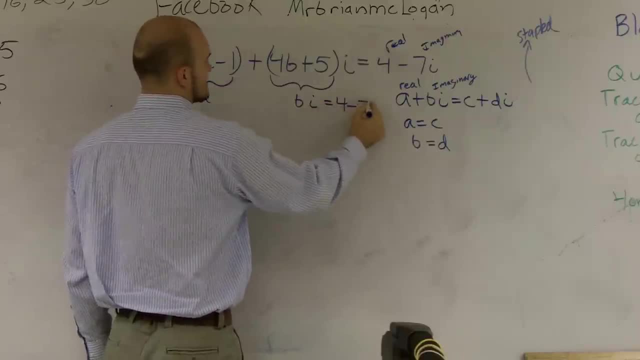 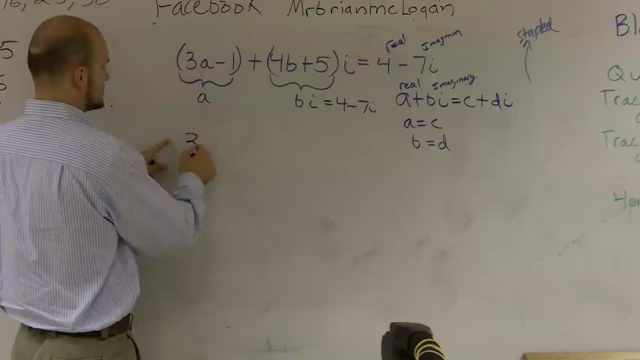 But if you can make this your b and you multiply that by ia, it would become 4 minus 7i, Where 4 is your real. so this, so therefore, you have two equations You could say: 3a minus 1 has to equal 4.. 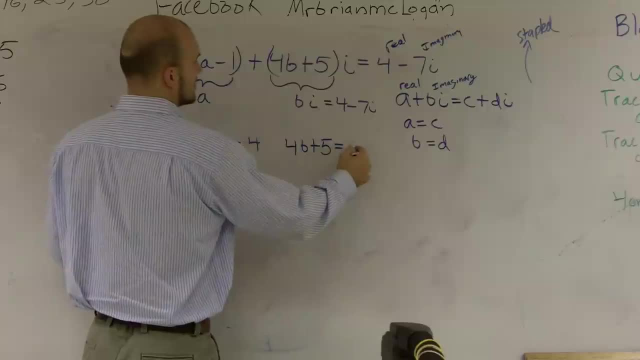 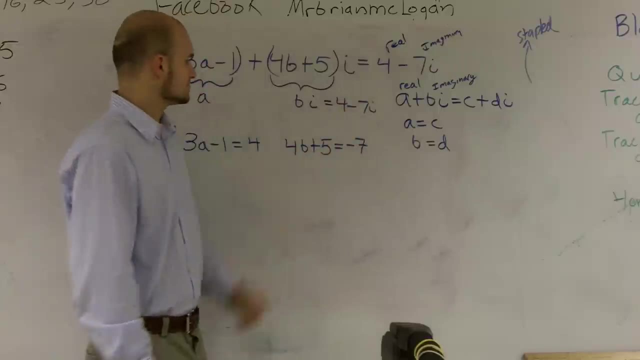 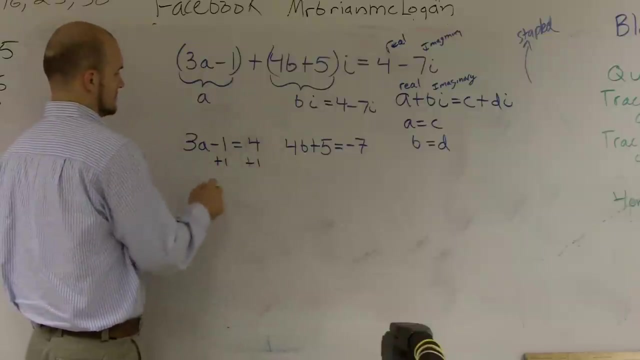 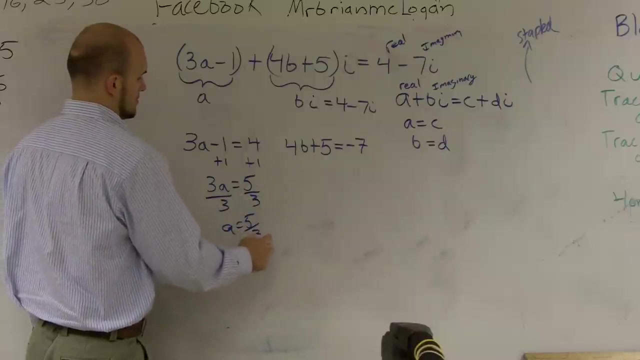 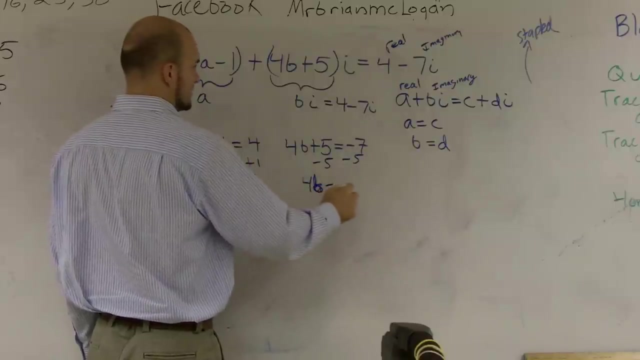 And you can say: 4b plus 5 has to equal a negative 7.. Because a has to equal c and b has to equal d, Does that make sense of two linear equations that we have to solve for? So I have to say: plus 1, 4b equals a negative 12.. 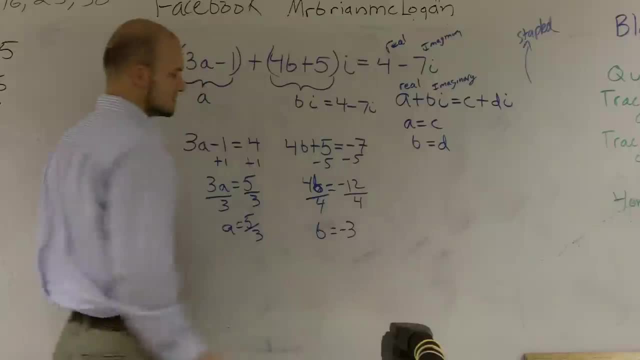 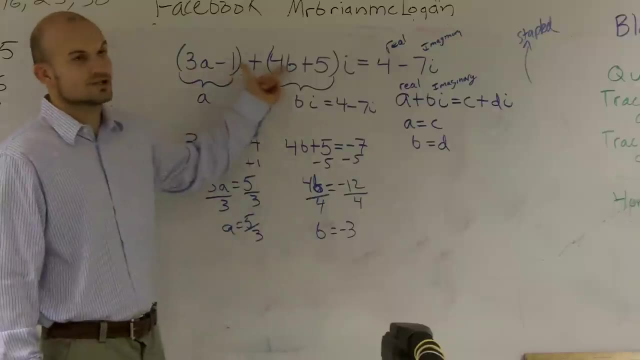 Divide by 4, b equals a negative 3.. So therefore the values for a and b have to be a: 5 thirds and a negative 3 for these two complex numbers to equal each other. OK, Good. 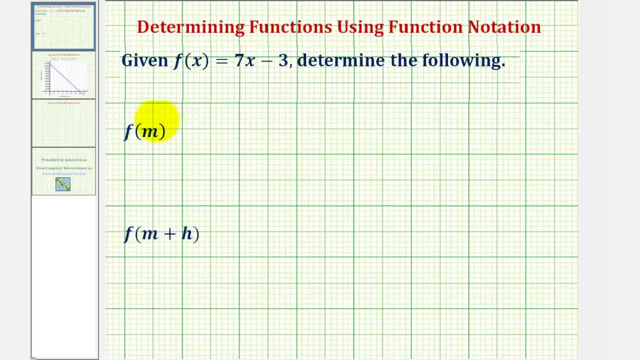 We're given, f of x equals seven x minus three. We want to determine f of m and f of the quantity m plus h. So for f of m, notice how the input is m, which means we'll substitute m for x in f of x. 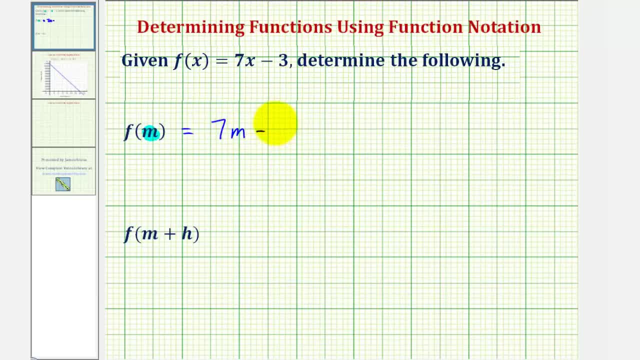 So we would have seven m minus three, which means when the input is m, the output is seven m minus three. Also notice: f of m is a function of m rather than a function of x. And now for f of the quantity m plus h. 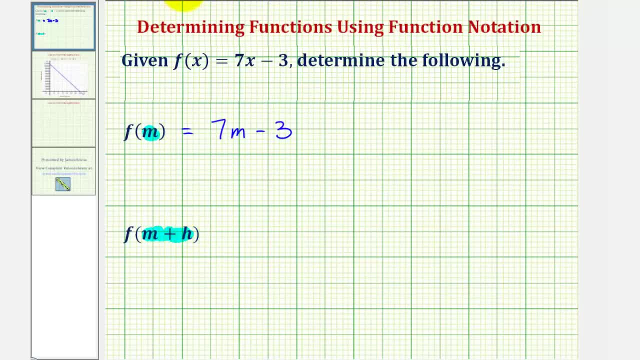 we'll substitute m plus h for x, since m plus h is our input. So we would have seven times the quantity m plus h minus three. And now we'll clear the parentheses by distributing here: So f of the quantity m plus h is equal to seven m plus seven h minus three.